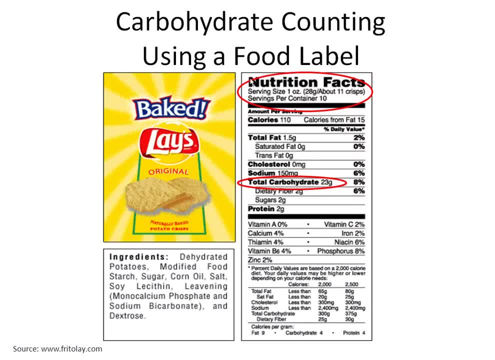 The serving size listed on this label is one ounce. You may be asking yourself: what does one ounce look like? You can next look at this and find that the weight of one ounce, or 28 grams, is about 11 crisps. 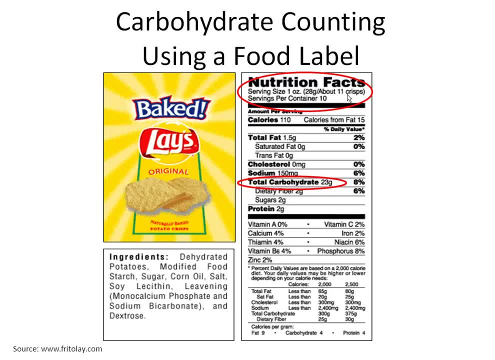 We all know that these crisps can be broken in the bag and it may be difficult to count out 11 crisps, So we recommend for you to use a food scale for accurate carbohydrate. If you weigh the crisps on a food scale, you can weigh it either in ounces or in grams. 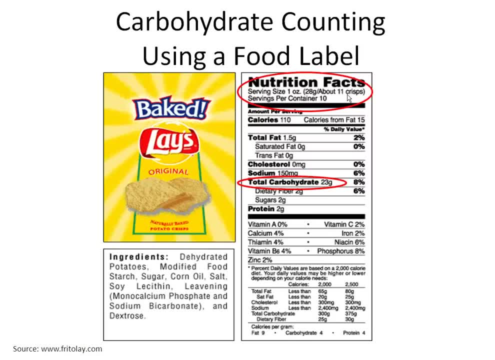 Remember the weight in grams is not the grams of food, It is the grams of carbohydrate. Once you have weighed one ounce of crisps, you can look further down on the food label to find the total grams of carbohydrate, The grams counted here. one ounce of crisps equals 23 grams of carbohydrate. 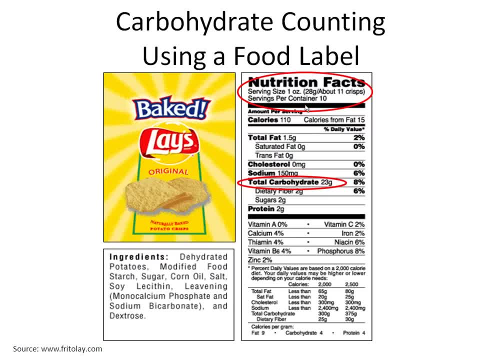 This bag of crisps contains 10 servings. So if you eat more than one serving, you are eating more than 23 grams of carbohydrate. For example, if you eat two ounces, you are eating 46 grams of carbohydrate. If you double the portion size, you need to double the total carbohydrate grams. 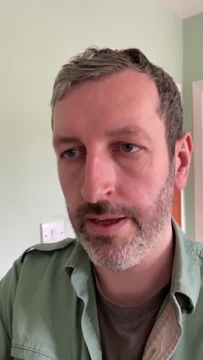 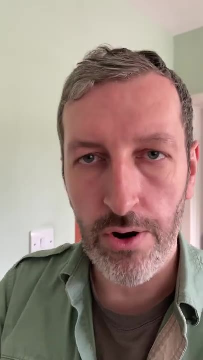 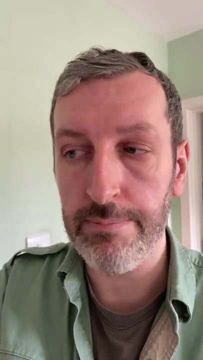 I am about to show you how to measure your height properly. Do not measure your height like Ra Pal. End of quote. Firstly, take a pen or a paper mate pencil. Secondly, an aerosol can, Preferably curved, like my ladies. Thirdly, tape measure. Fourthly, no socks.